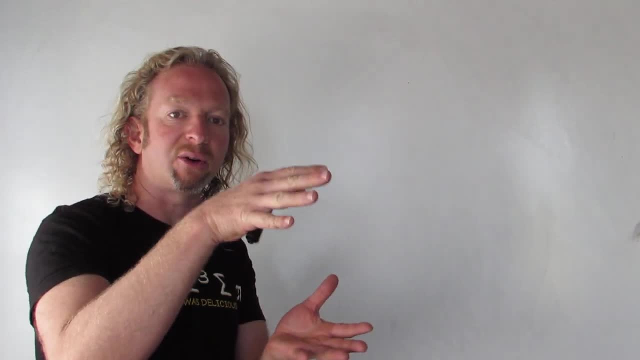 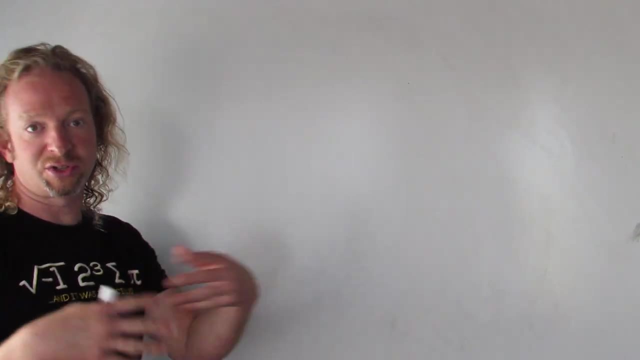 derivative of that function will tell you how hot the room is getting or how cold the room is getting, So how fast it's heating up or how fast it's cooling down. So limits are used for derivatives which describe rates of change. In this video, we're going to talk about the notation behind limits. okay, 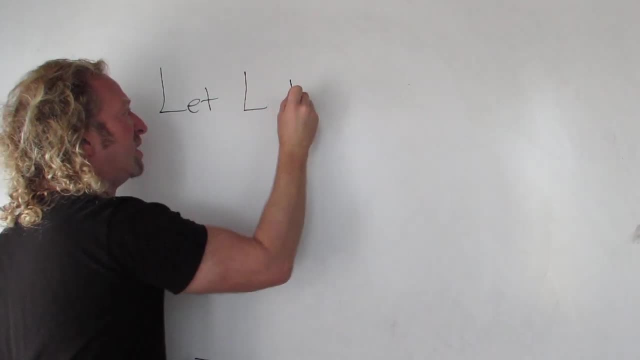 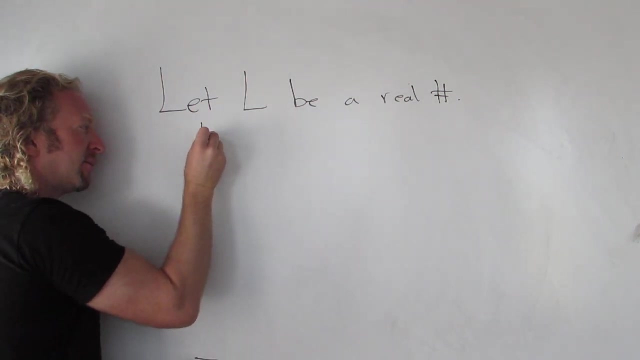 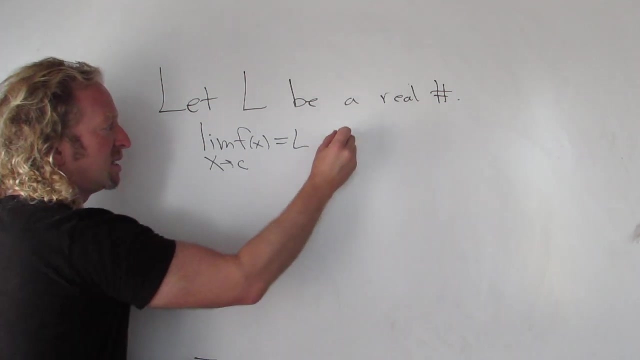 So let big L be a real number. So be a real number. So this is the limit notation. So you write Lm. So the limit of f of x as x approaches c is equal to L. So this is read: the limit of f of x as x approaches c is equal to L. So this means, so means. 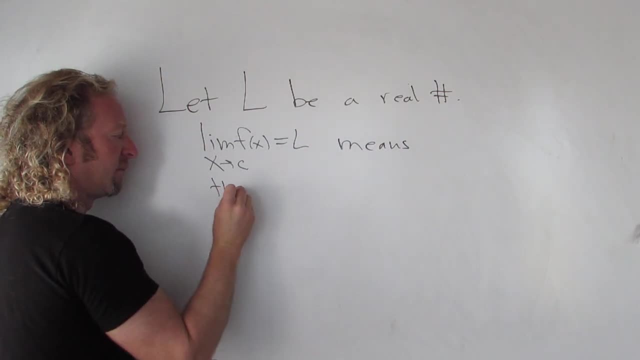 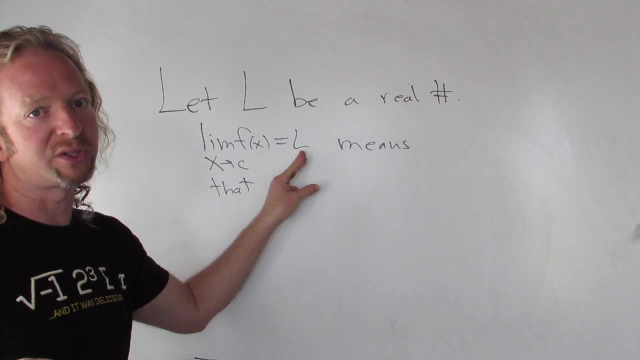 that. well, it basically means that whenever x gets really really, really really close to c, f of x gets really really really really close to L. Remember, f of x is the y value, So when the x value gets close to c, 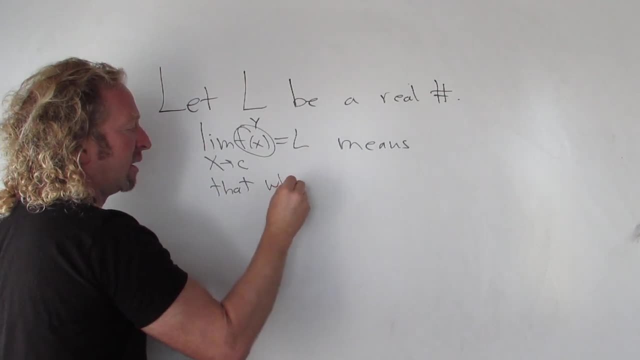 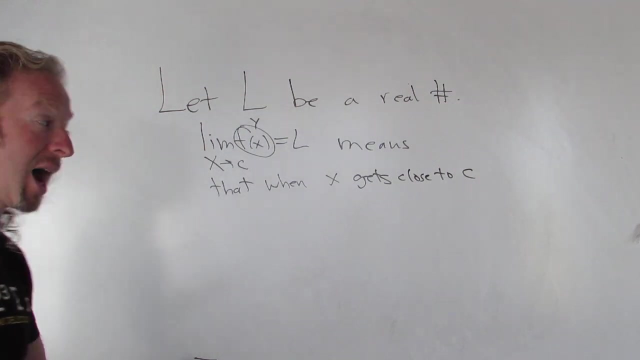 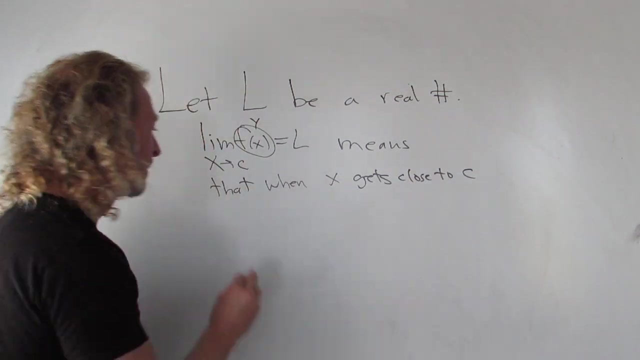 the y value gets close to L Means that when x gets close to c, you might say: what does close mean? Ah, So how close, As close as you like, right, You can literally get as close as you like. So when x gets close to c, f of x. 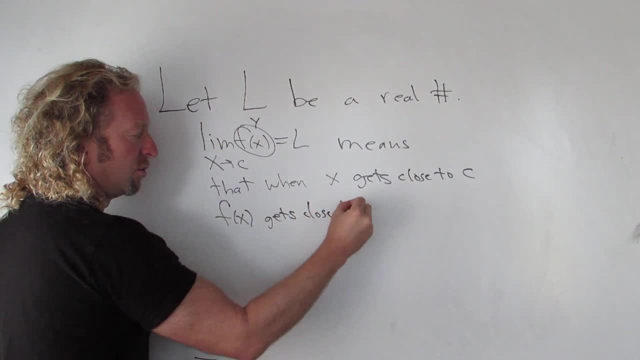 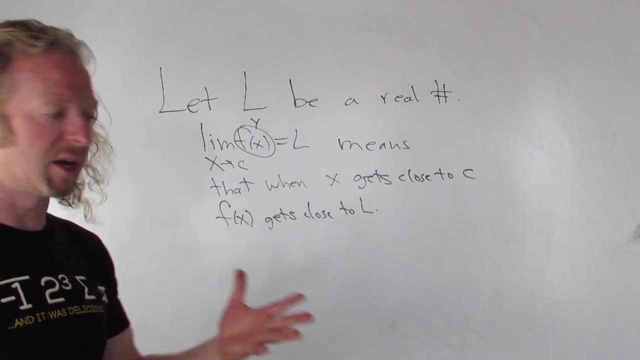 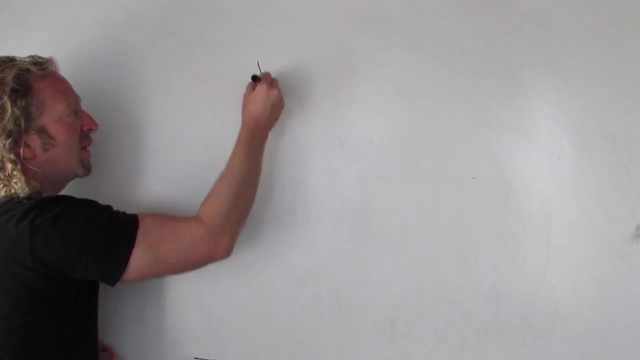 gets close to L. Maybe now we should do a simple example of limits So you can see what it means intuitively and so you can see what it means graphically. I think I have something here to erase, so let's do it. Let's draw a quick graph, Say: we have 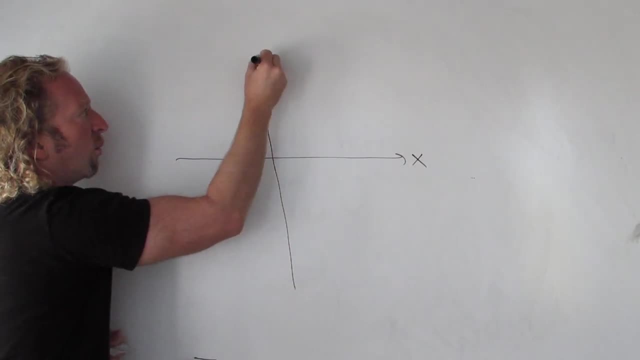 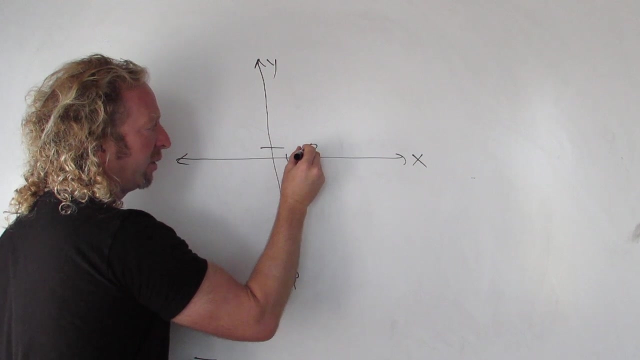 the y-axis and say we have the x-axis, So x, y. Let's make up some numbers, let's see So like one, two, three, one, and I'll put a little hole here and I'll come down here, go through three. 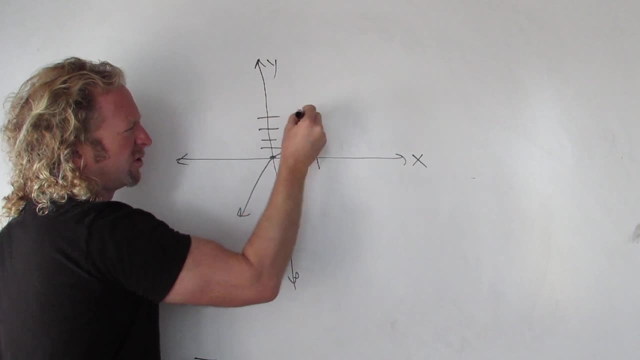 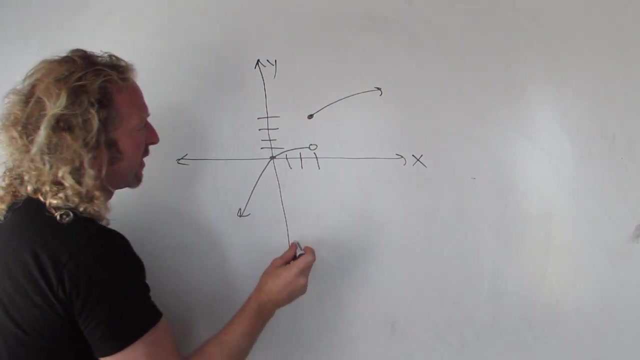 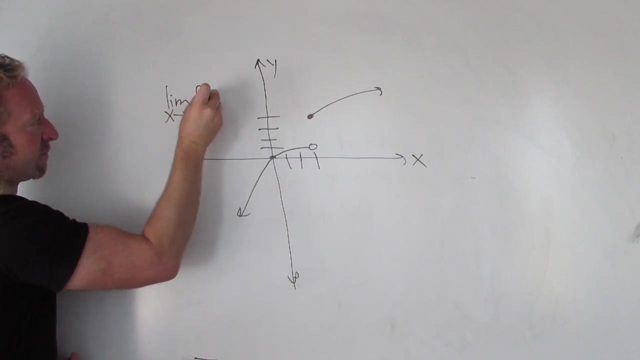 0 and come up here 1, 2, 3, 4, just use different numbers and that's good, okay. so let's compute some limits. let's do it. so first let's find the limit as X approaches 0 of f of x. so this is asking: what happens to the Y value when X gets? 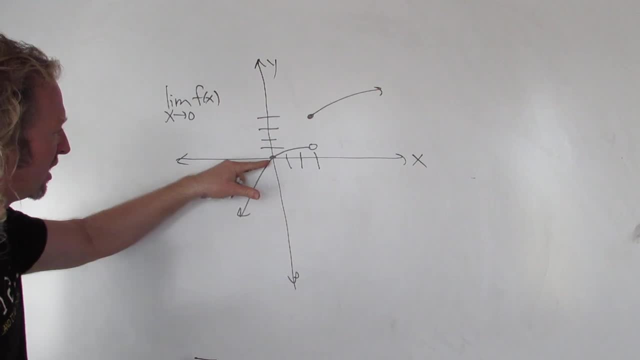 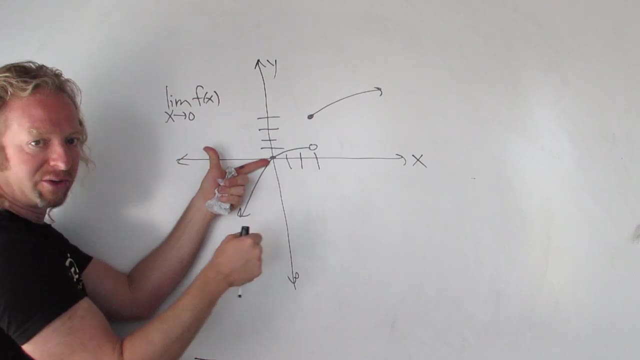 close to 0. so the idea is this: you want to approach 0 from both directions. okay, from the left and from the right. so when X is close to 0 from the left, the Y value is 0. when X gets close to 0 from the right, the Y value is 0. therefore, the 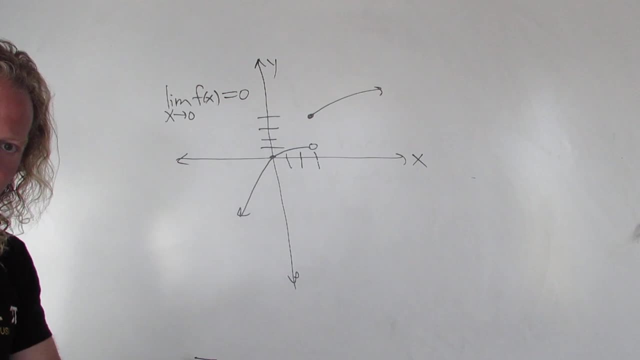 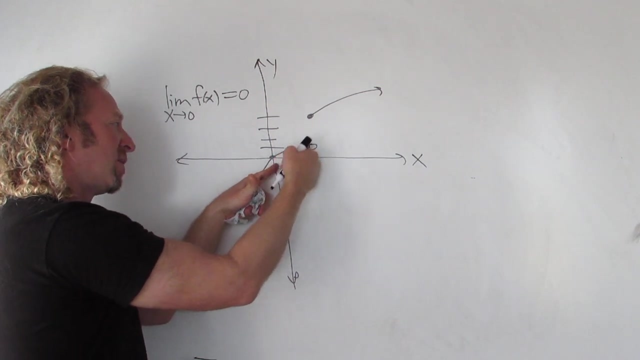 limit is zero, so you have to be able to approach from both directions to get an answer. so, as X approaches zero from the left, the Y value approaches 0. as X approaches 0 from the right, the Y value approaches 0. therefore, the limit is 0. 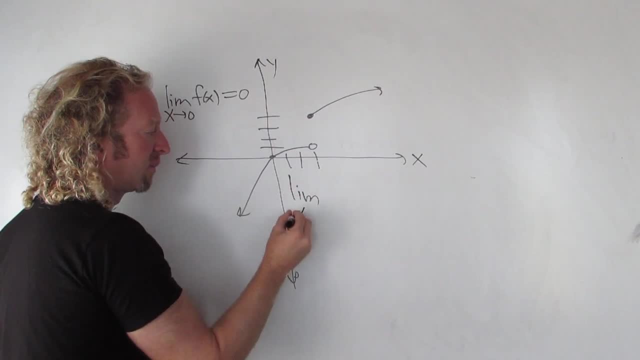 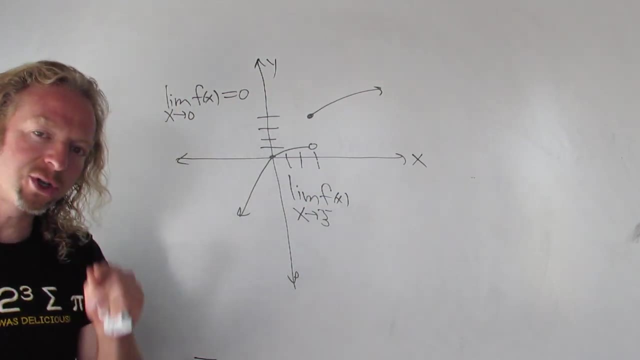 let's look at approaching 3. let's approach 3. however, I'm going to put a little negative sign here. so this negative sign means we're approaching only from the left. okay, if you put a plus sign means you're approaching from the right. so we're approaching three from the left. so as 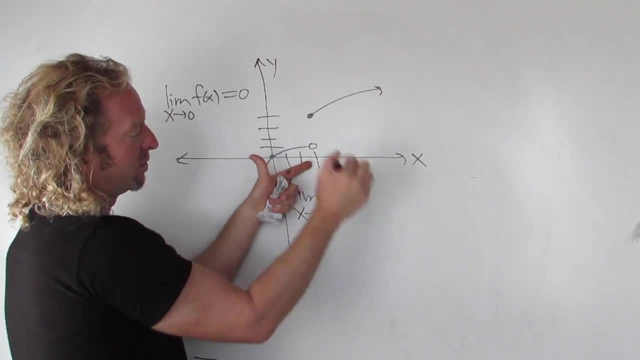 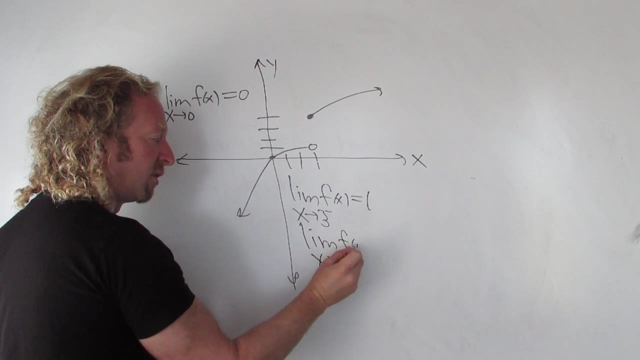 the X value approaches three from the left. looks like the Y value is one, but now let's approach three from the right. so we use the plus sign for that. so, as X approaches three from the right, let's see what happens. so here's, here's X. 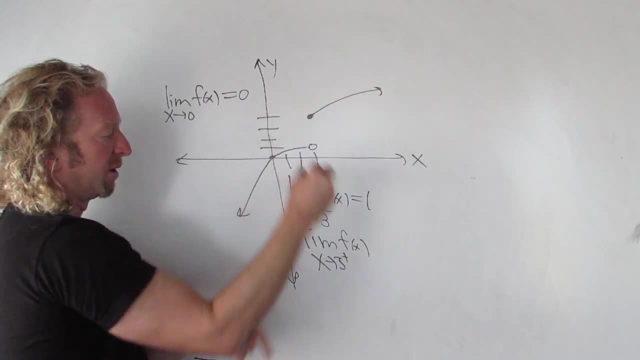 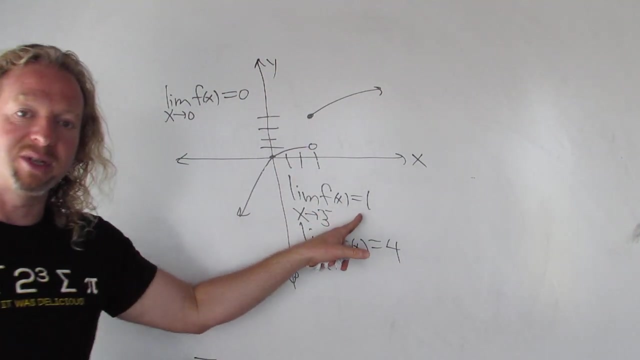 it's approaching three so the Y value is close to one. two, three, four. so when you approach three from the left right the X value gets really really close to three. the Y value gets close to one. so we said the limit is one as X approaches three. 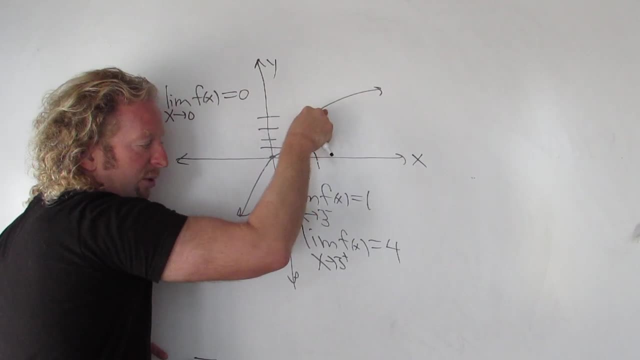 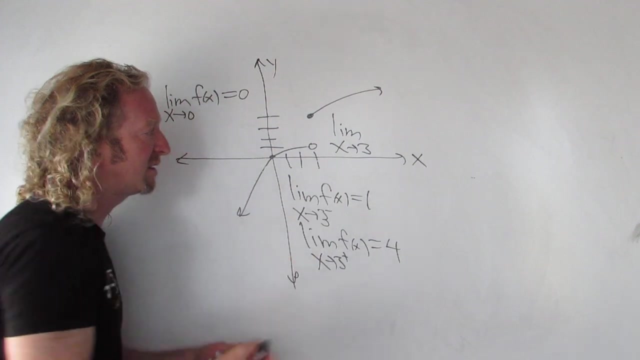 from the right, the Y value gets really, really, really, really really close to four. so we say the limit is four. so what would that mean in terms of the limit? well, that means that the regular limit- you can think of this as a two sided limit, usually called one sided limits- the regular limit is for both directions. 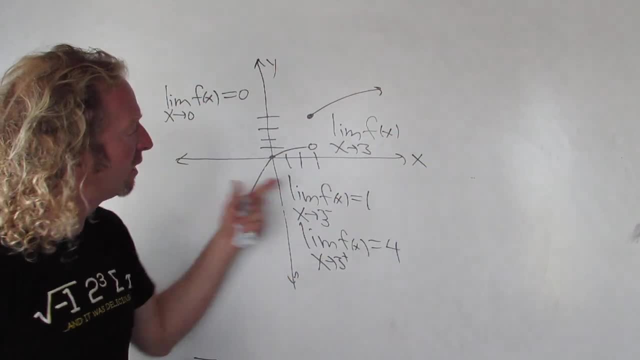 so as X approaches 3, well, from the left we get 1, from the right we get 4. therefore we get nomenclature in the rules. use唇 when we're approaches three. Let me whack these two zoom erosions answer when we approach from both directions. so in this case you would say: 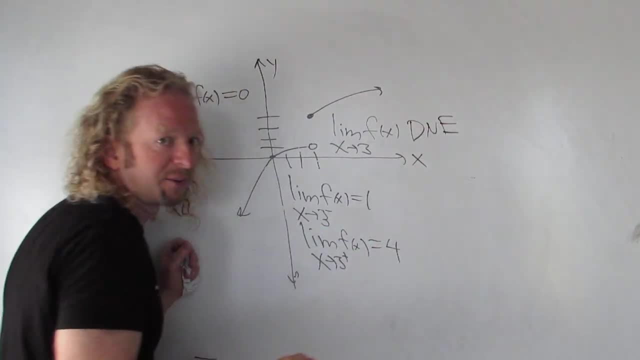 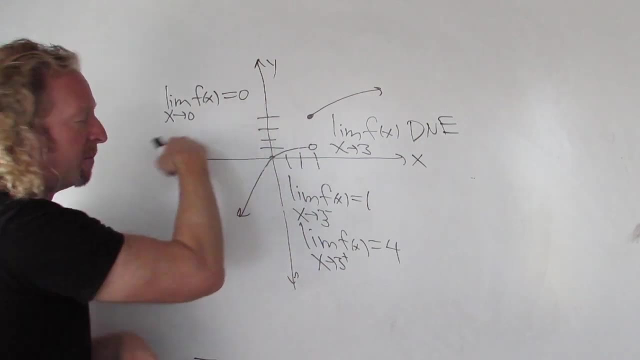 the limit D and E, and that means does not exist in this example. here I didn't use one-sided limits. I just showed you: from the left you get zero, from the right you get zero. therefore, the limit is zero. if you wanted to write it formally, you'd write the limit as X approaches zero from the left or from.